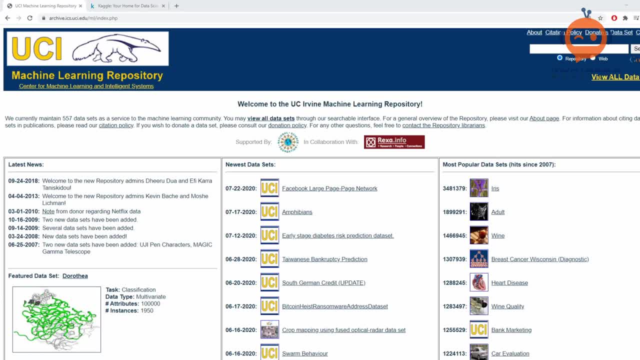 Hey everyone, welcome to my channel. In this video we will use real-world data to create a multi-linear regression model to predict the rent of houses. The input attributes will include the number of rooms, the number of bathrooms, the parking spaces and more. We will first look at where we can get this data from and 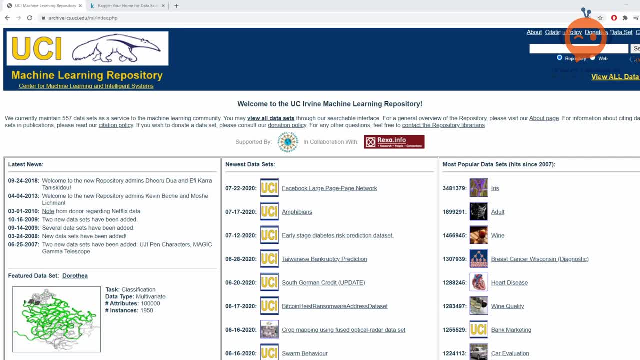 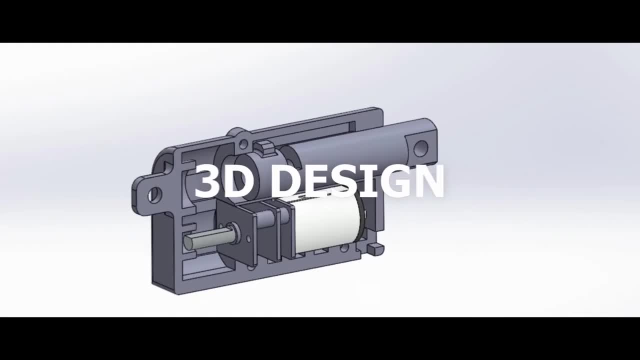 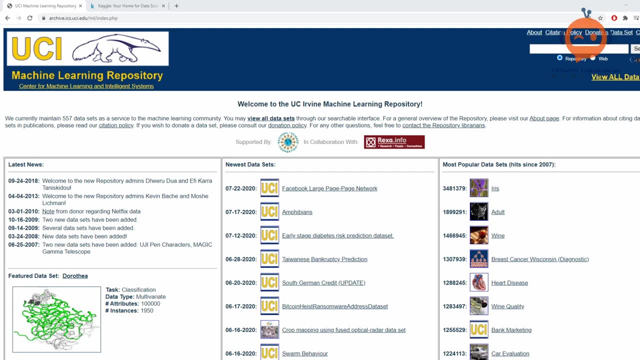 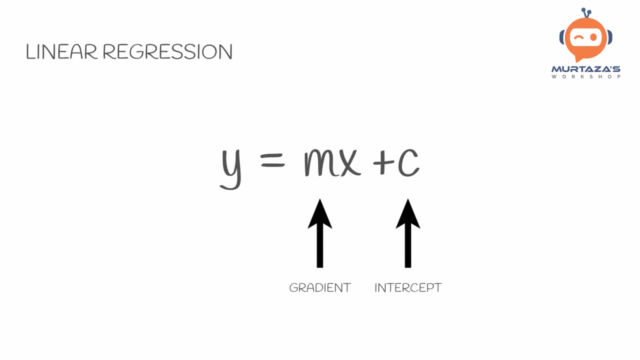 then how we can clean it up to feed it to the linear model. So let's get started. So in the previous video we saw the concept of linear regression, which was y equals mx plus c. So we had one gradient and we had one intercept. So the idea here is that now we have multiple 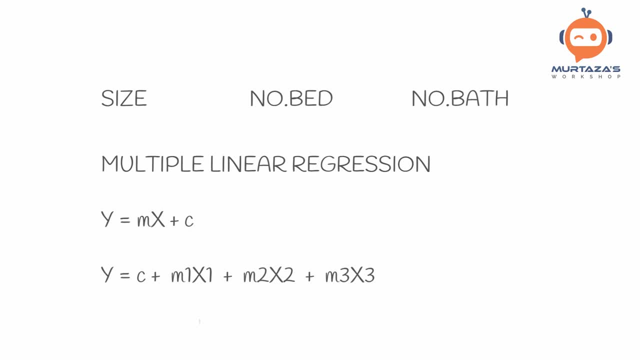 linear regression. so therefore we will have multiple gradients, or you can say multiple slopes, but we will have only one intercept. So if you are not familiar with this concept, you can go back and check out the theory part where I explained all of this in detail. 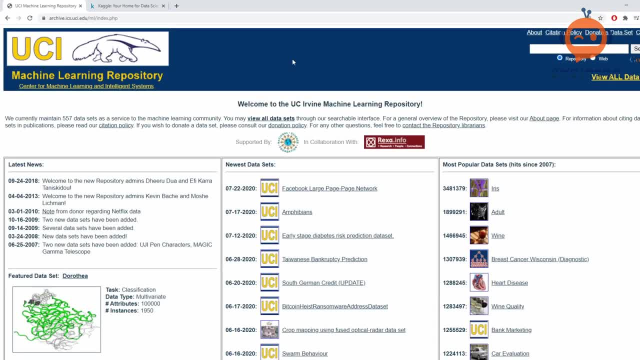 So before starting any machine learning problem, we need to find the data. So there are multiple resources where you can get this data from. You can generate your own data as well, but two places that I highly recommend to check out are the UCI machine learning repository and the other one is 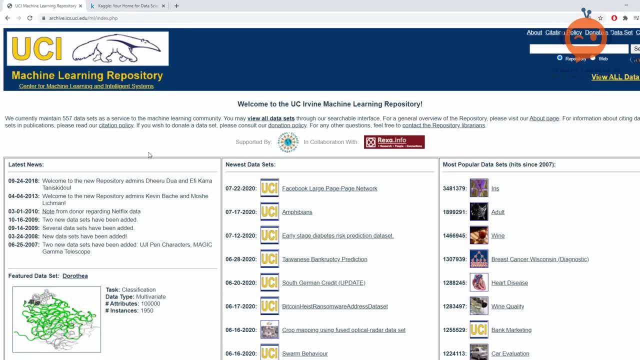 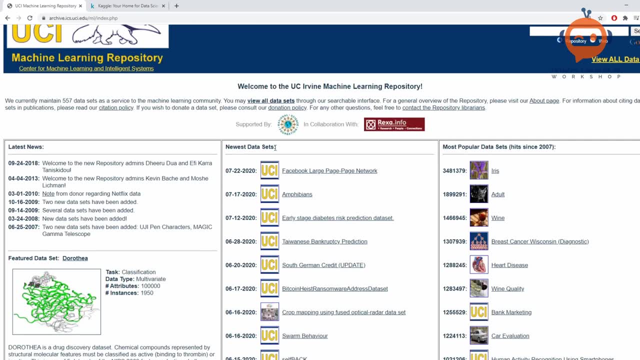 Kaggle. So let's have a look at UCI. So if we go here and we look at these different data sets- and these are the ones that are, these are here the newest ones and here we have the most popular data sets since 2007- and if we click on view all data sets, then we can see here that we have. 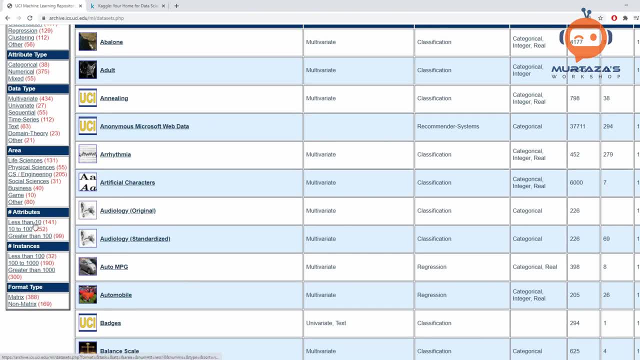 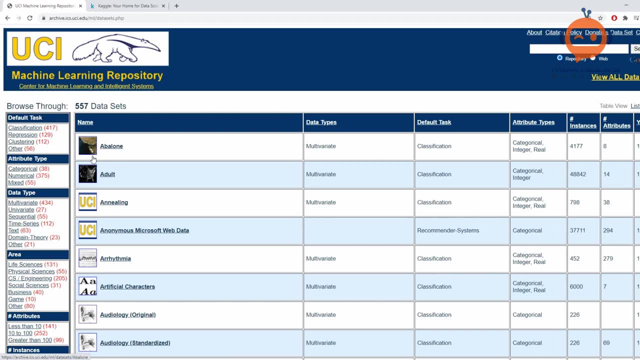 lots of categories where we can select our relative data. Now the thing is that, if you have seen the previous videos, we discussed about the categories of problems, so here they have defined those. so if we are talking about supervised, we have problem types of classification and regression, and if you are talking about unsupervised, then we have clustering and 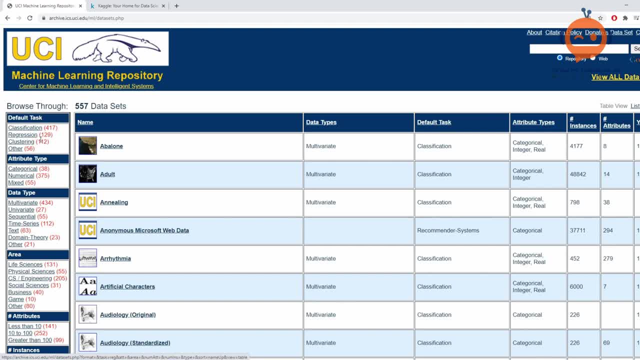 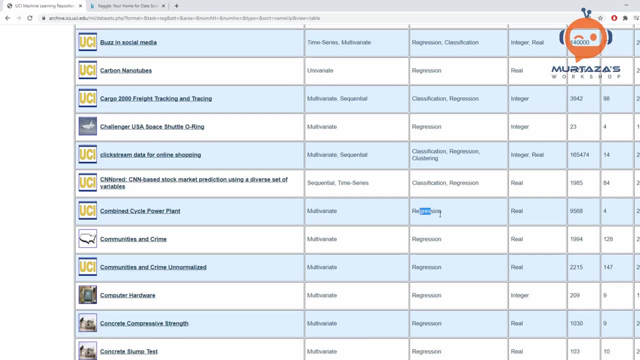 association problems. So here you can see that they have sorted these out. so, for example, in this case we want multiple linear regression, so it is regression, so we will click on regression. So here we can see that we have all the data sets that are related to regression. so you can see here. 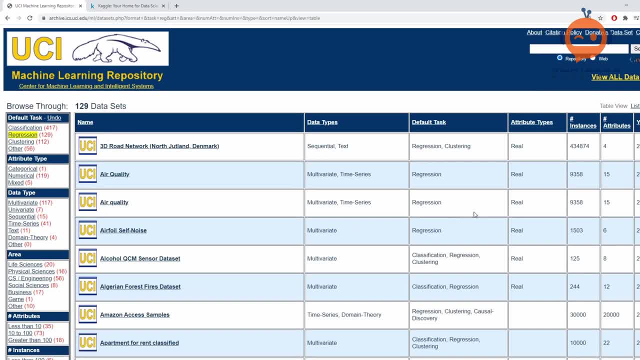 these are all the regression types. so here we can see that we have two main things which are basically your instances and your attributes. so instances are basically, if we are talking about houses, then how much data we have or how many houses we have. so, for example, if we 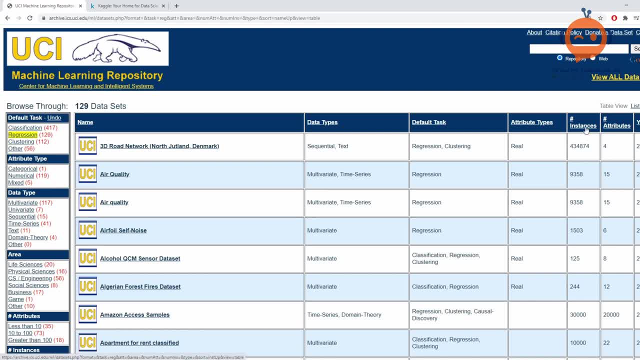 have data of a hundred houses, so the instances will be hundred and the attributes are basically the features. so, for example, the number of rooms is one feature, then the number of bathrooms is one feature, the parking spaces in is one feature. so how many features do we have? these are basically your attributes. in other words, you can call attributes. 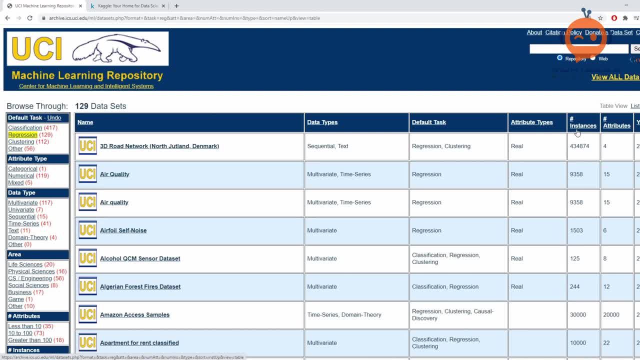 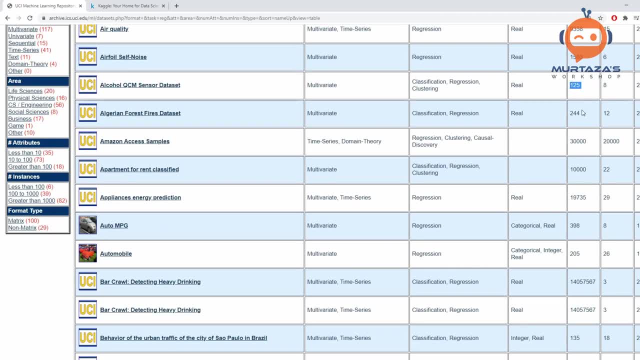 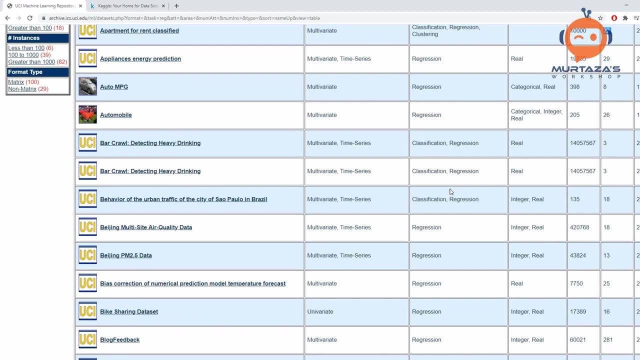 your columns and your instances, your rows. so here you can see that this is quite a large data set. here you have small ones, 125, and here you have 10,000 with 22 attributes. so you can find different data sets with different instances and different attributes. so the one we are going to use today 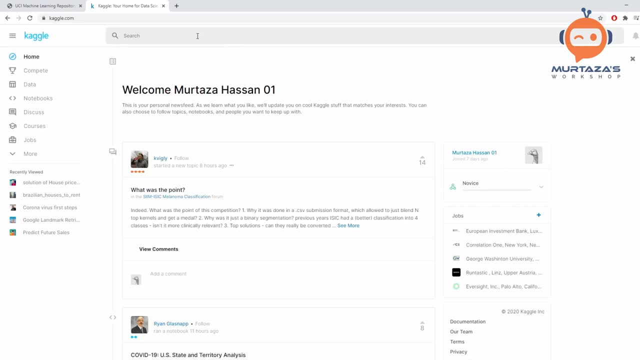 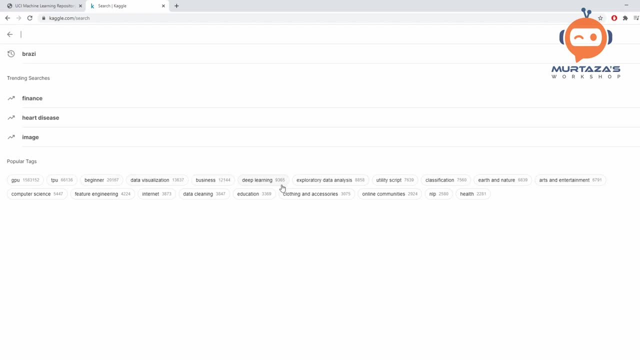 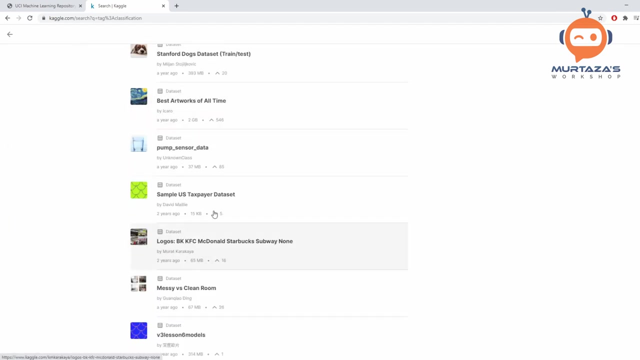 is through Kaggle and if I go here- and, by the way, the same thing goes with Kaggle- you have these tags that you can use. so, for example, I can click on classification and I will find all the data sets that are available for classification, so I can click in on any one of. 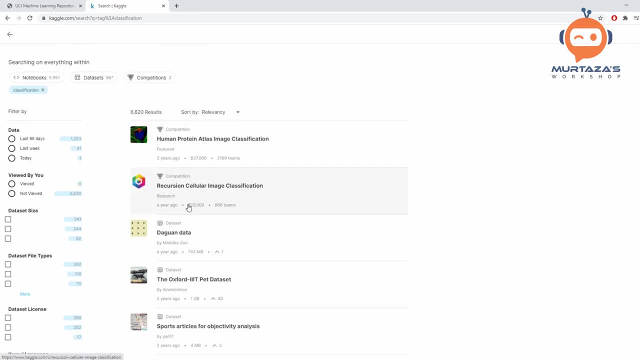 these and I can use them, and some of them are basically part of a competition that have prices as well anyways. so the- the one that we are using today- is basically for rent, so we will write here: house rent and this is the Brazilian house to rent data set that we will be using. 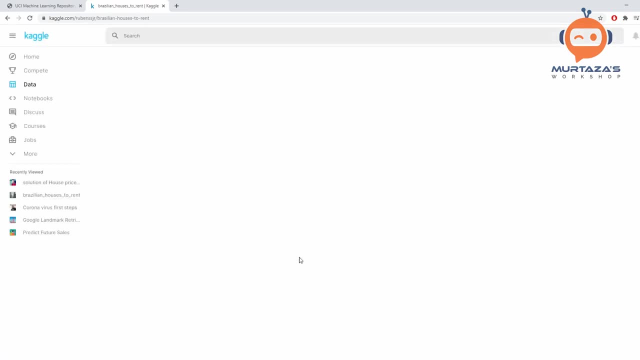 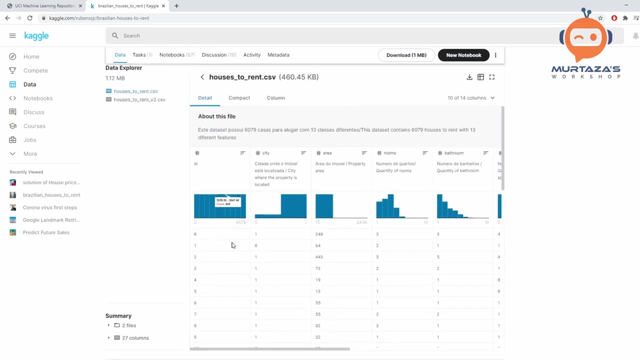 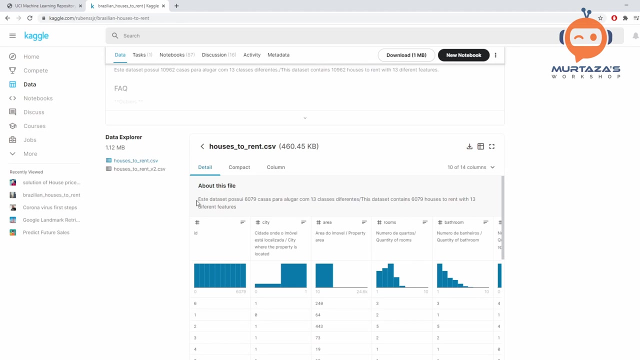 so let me click on that and there we have the data sets. here you can see that we have- this is the actual files that we can download- houses to rent. houses to rent- version two, and here you can see that we have these different attributes. so you have the city, you have area. 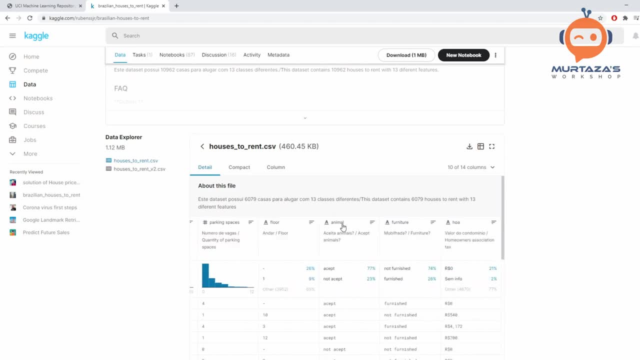 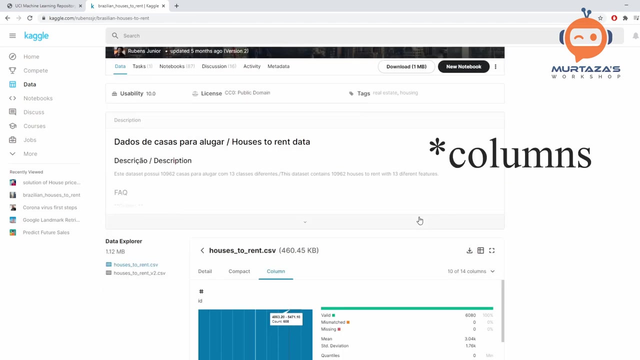 you have number of rooms, number of bathrooms and you can scroll and you can see how many which floor number. we have. animals, if they are allowed or not, furniture, so if we go to column and then we can see how much do we have for each one of these. so we will not be using all of them. we will be using. 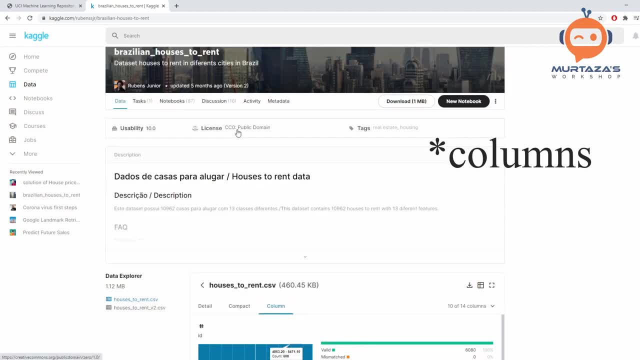 some of them to actually create our model. so before you actually download or use any data set, just make sure you understand the license. so here is the uh declaration of the license. so this one is basically Creative Commons zero and it is public domain. so here we can download. if I click on that, it will start the 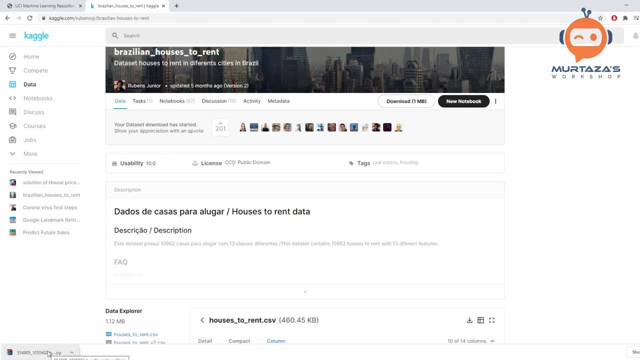 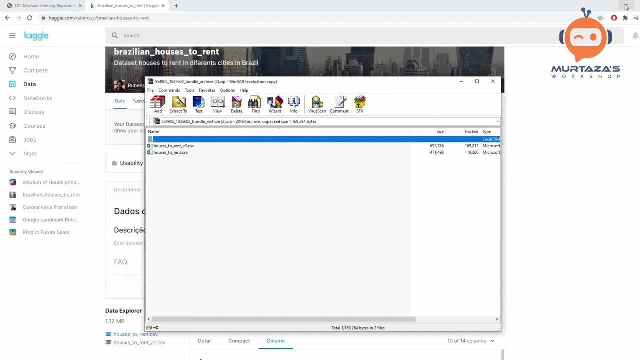 download and because this is small file, it will download relatively quickly. so I can click on that. and here we have- let me close that- and here we have the files. so we have houses to rent and houses to rent version 2, so I will be using houses. 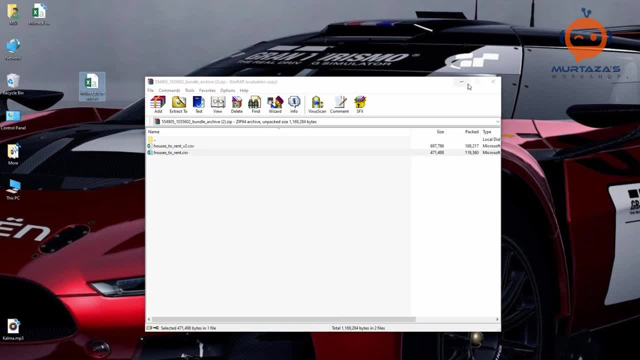 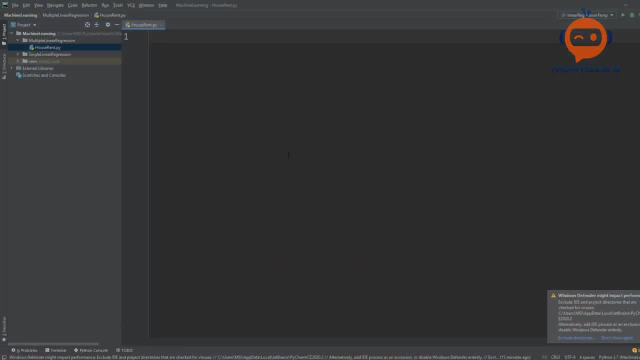 to rent rather than houses to rent- version 2. so I will open up. I will open up PyCharm, and here we have a new project. actually, this is the one that we did with linear, single linear regression as well. so we have already installed the relevant libraries, but I will show you how you can do that. then, here we have. 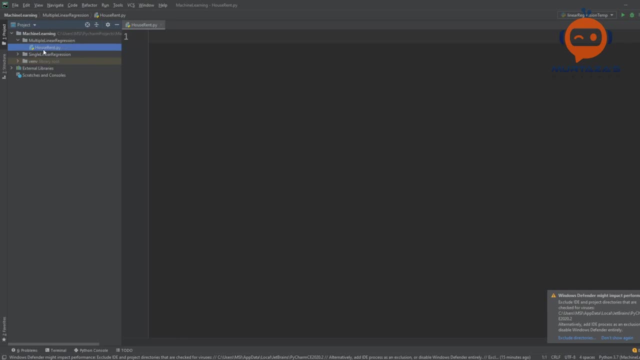 the multi linear regression folder and then inside that we have the multi linear regression folder, and then inside that we have the multi linear regression folder, and then inside that we have the house rent as our pie file. so this is house rent as our pie file. so this is the main file. so all you have to do is you. 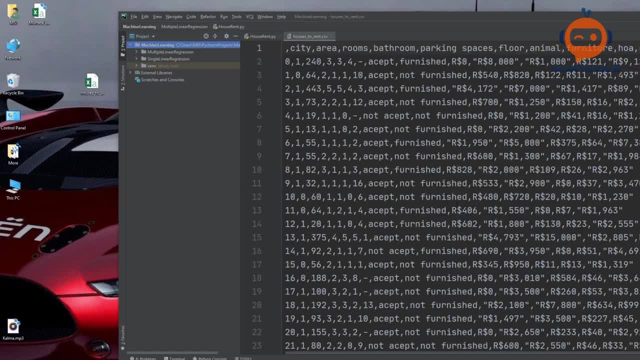 the main file. so all you have to do is you have to just drag and drop into the have to just drag and drop into the folder and just click OK. and here we folder and just click OK, and here we have the data set. now so you can see. 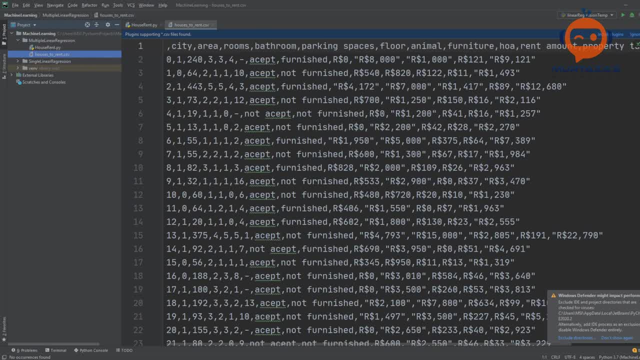 have the data set now, so you can see houses to rent, and so these are houses to rent, and so these are basically CSV files, which means comma, basically CSV files, which means comma: separated values. so each value is separated values, so each value is separated with a comma, so you can see it. 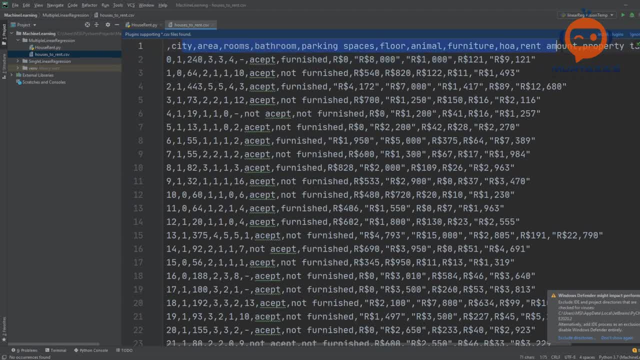 separated with a comma. so you can see it here and at the top we have the headings here and at the top we have the headings that we can use, that we can use and we can sort out our columns. so if I and we can sort out our columns, so if I say city, it will take all of this the 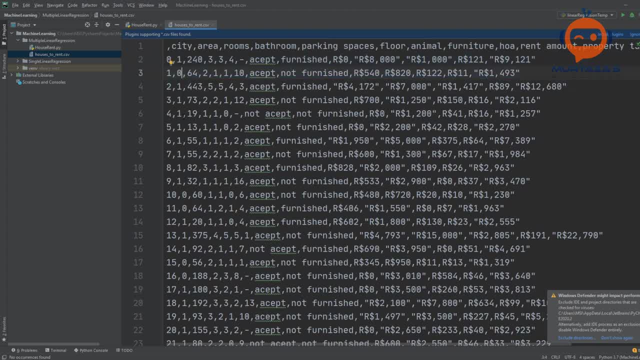 say city, it will take all of this, the second column, which is 1 0, 1 0 0, so all second column, which is 1 0, 1 0 0. so all of this basically tells whether it's a of. this basically tells whether it's a city or not. area is basically the number. 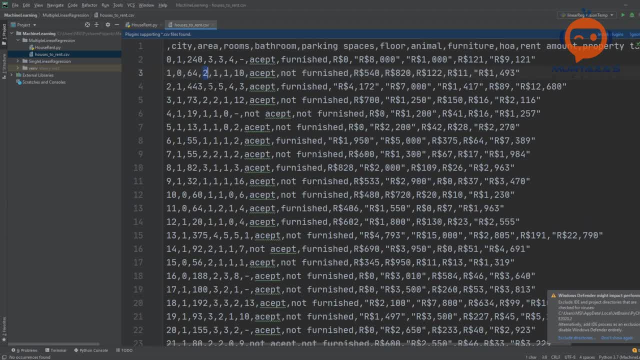 city or not. area is basically the number, the size rooms. you have three, you have the size rooms. you have three. you have two, you have five and then you have for two. you have five and then you have, for example, animal: it's accepted or not, so example: animal: it's accepted or not, so here you have not accepted, here you have. 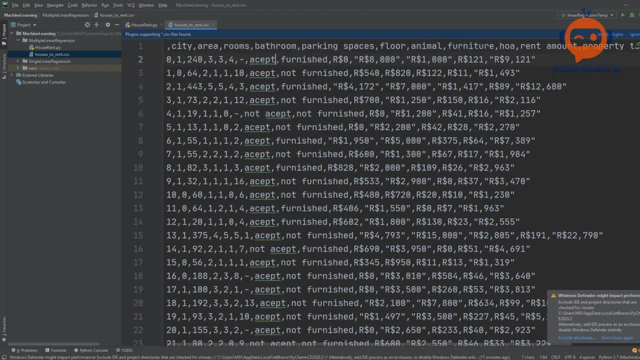 here you have not accepted, here you have accepted. and then we have the first accepted, and then we have the first column, and then we have the second column, and then we have the first column, and then we have the second column. furniture, whether it's furnished or not. 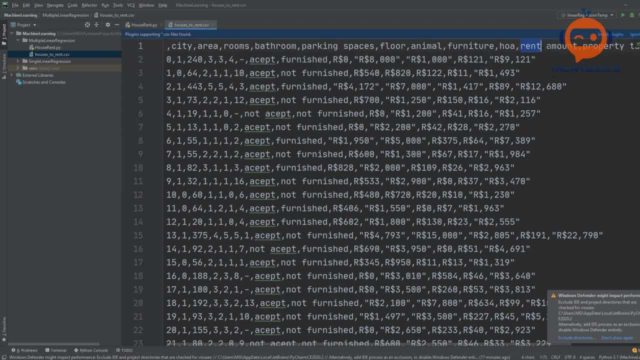 furniture, whether it's furnished or not. furniture, whether it's furnished or not furnished, and then we have the rent the furnished, and then we have the rent the furnished, and then we have the rent the rent amount. this is the value that we rent amount. this is the value that we 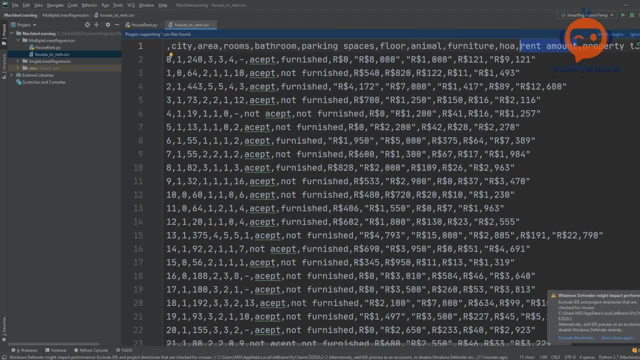 rent amount. this is the value that we will be trying to predict. so you can see. will be trying to predict. so you can see, will be trying to predict. so you can see here- I'm not sure which one of these here. I'm not sure which one of these. 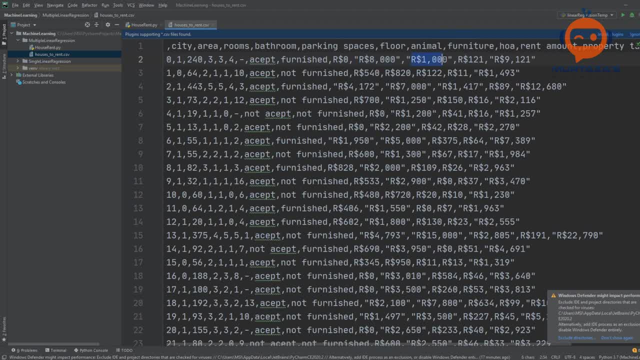 here. I'm not sure which one of these: this is probably this one. and then we: this is probably this one, and then we: this is probably this one. and then we have some other values as well. now the have some other values as well. now the have some other values as well. now, the thing is that they have, they have made. 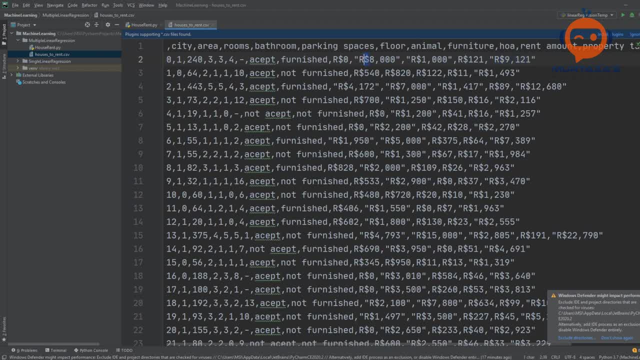 thing is that they have. they have made thing is that they have. they have made it a little bit difficult to use this. it a little bit difficult to use this. it a little bit difficult to use this because they have added this R and because they have added this R and. 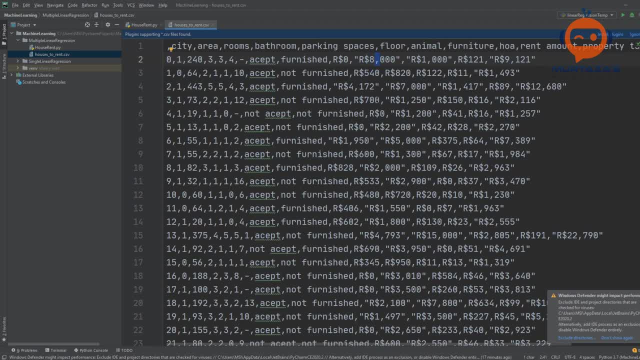 because they have added this R and dollar in front and they have commas and dollar in front and they have commas and dollar in front and they have commas, and we will have to filter all of this out. we will have to filter all of this out. we will have to filter all of this out, but it's not that difficult, it's it's. 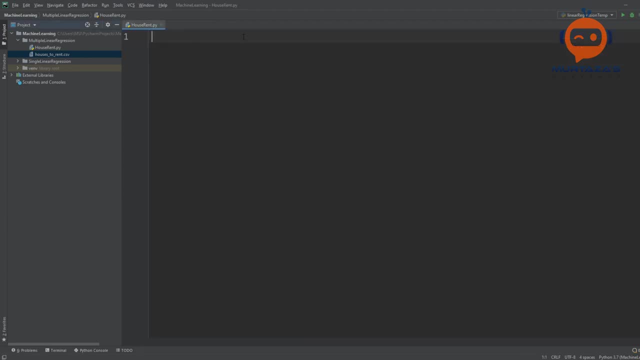 but it's not that difficult it's. it's, but it's not that difficult, it's. it's not something big, so we will be able to- not something big, so we will be able to- not something big, so we will be able to solve that problem. so the first thing is: 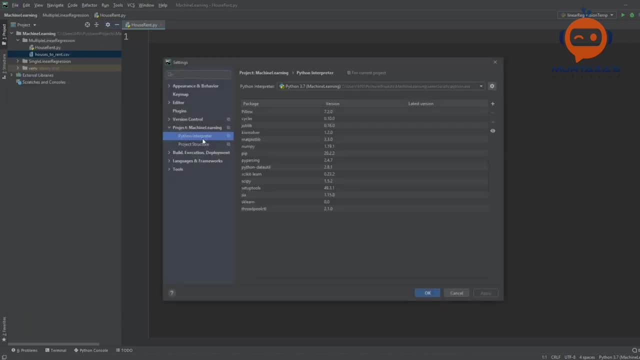 solve that problem. so the first thing is: solve that problem. so the first thing is: again you will go to files, you will go again. you will go to files, you will go again you will go to files. you will go to settings and here in the interpreter, to settings and here in the interpreter. 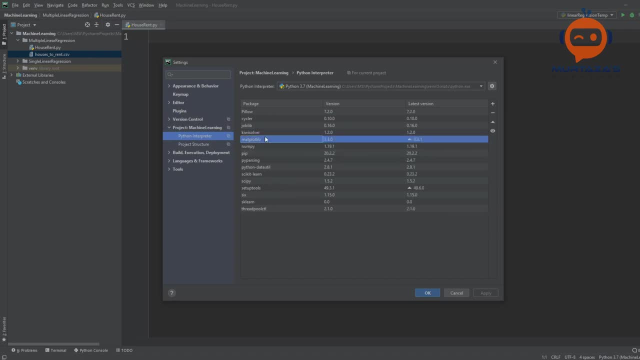 to settings and here in the interpreter, you are going to install, you can. you are going to install, you can. you are going to install. you can install matplotlib. I don't think we will install matplotlib. I don't think we will install matplotlib. I don't think we will be using this. then you will have to. 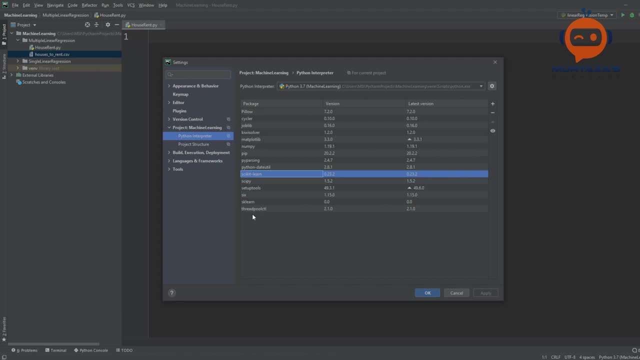 be using this, then you will have to be using this, then you will have to install scikit-learn, and then you have to install scikit-learn, and then you have to install scikit-learn, and then you have to install what else? I think that that is. install scikit-learn and then you have to install what else. I think that that is: install scikit-learn and then you have to install what else. I think that that is pretty much it. the rest are just the pretty much it. the rest are just the. 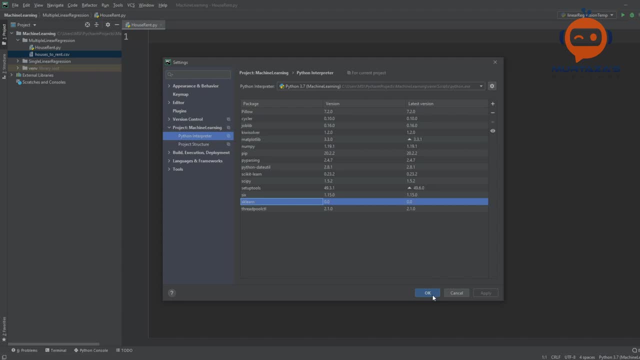 pretty much it. the rest are just the dependencies, and it will download or dependencies, and it will download or dependencies and it will download or install by itself. okay, yeah, one more install by itself. okay, yeah, one more install by itself. okay, yeah, one more thing we have to install. let's go back. 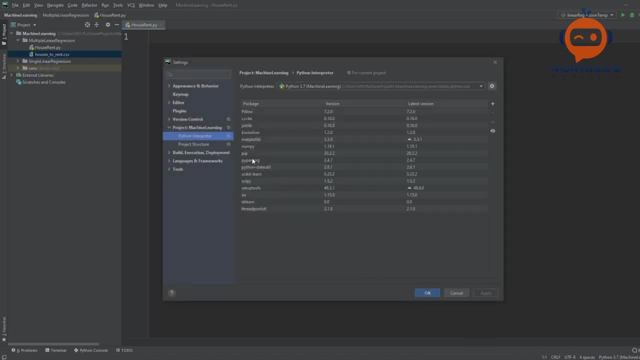 thing we have to install, let's go back. thing we have to install let's go back is pandas. is it here? I don't think so. so is pandas. is it here? I don't think so. so is pandas. is it here? I don't think so. so let's install pandas. 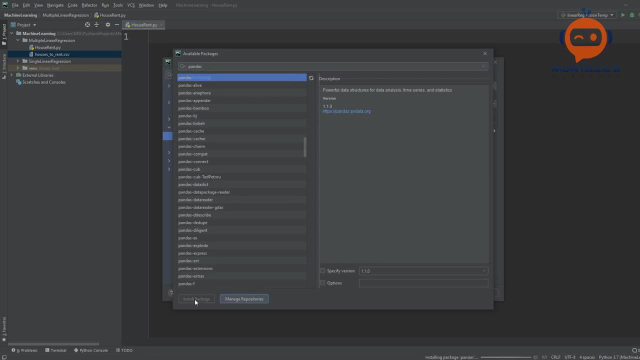 let's install pandas. let's install pandas. so pandas is the library that will allow so, pandas is the library that will allow. so pandas is the library that will allow us to get the data from our CSV file and us to get the data from our CSV file. and 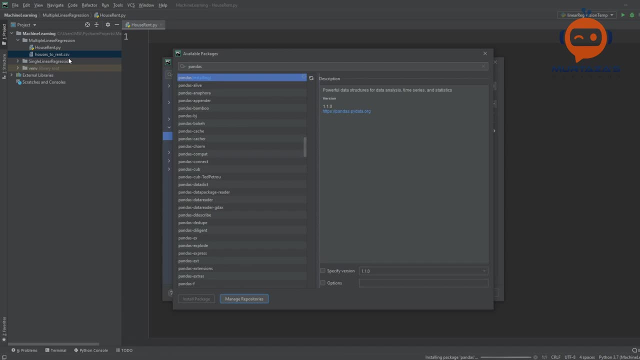 us to get the data from our CSV file and it has some built-in functions that will. it has some built-in functions that will. it has some built-in functions that will help us to actually filter out our data, help us to actually filter out our data, help us to actually filter out our data so that we can easily send our data to. 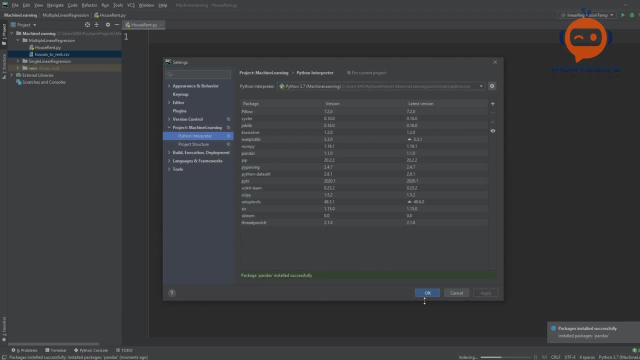 so that we can easily send our data to, so that we can easily send our data to our machine learning model. so it's a our machine learning model, so it's a our machine learning model. so it's a very useful library. so we are going to very useful library, so we are going to. 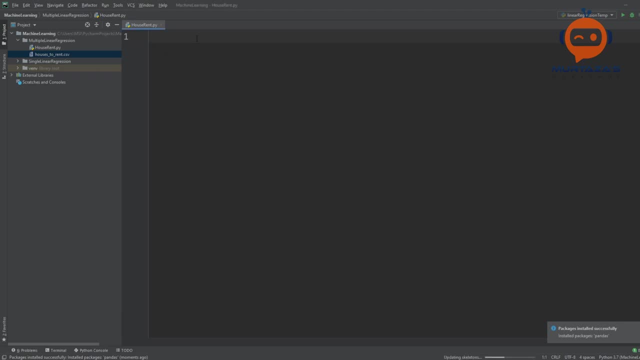 very useful library, so we are going to use that. so the thing is that whenever use that, so the thing is that whenever use that. so the thing is that whenever you are working with the data you can, you are working with the data you can, you are working with the data. you can use many different techniques to 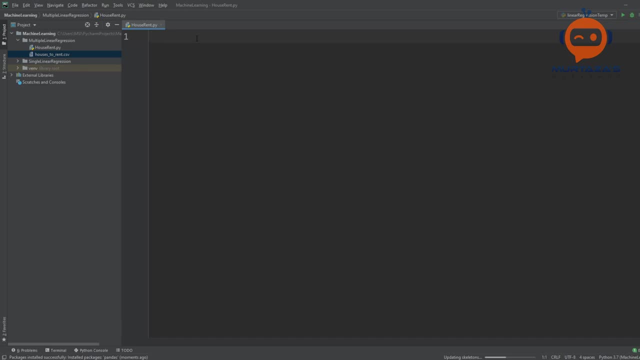 use many different techniques to use many different techniques to actually filter it out, make it cleaner, actually filter it out, make it cleaner, actually filter it out, make it cleaner. but the thing is that I recommend that. but the thing is that I recommend that, but the thing is that I recommend that you try to use limited amount of. 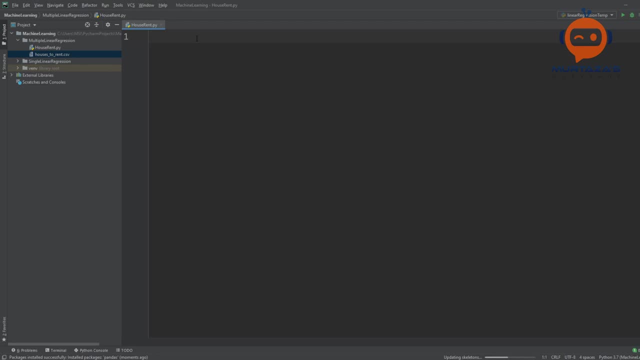 you try to use limited amount of. you try to use limited amount of libraries because there will be libraries, because there will be libraries, because there will be libraries that will allow you to perform libraries that will allow you to perform libraries that will allow you to perform actions very easily, but again, you don't. 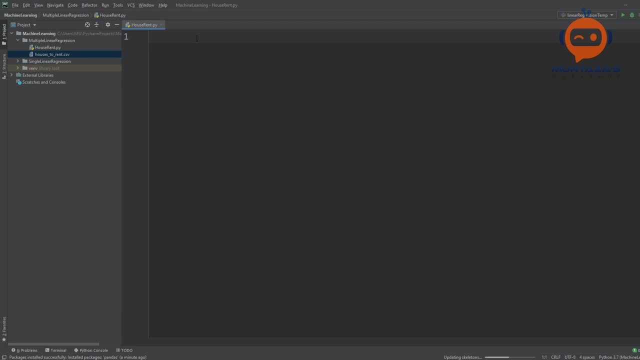 actions very easily, but again you don't actions very easily, but again you don't want to overdo it. so especially when want to overdo it, so especially when want to overdo it, so especially when you're starting. so I will try my best to you're starting, so I will try my best to. 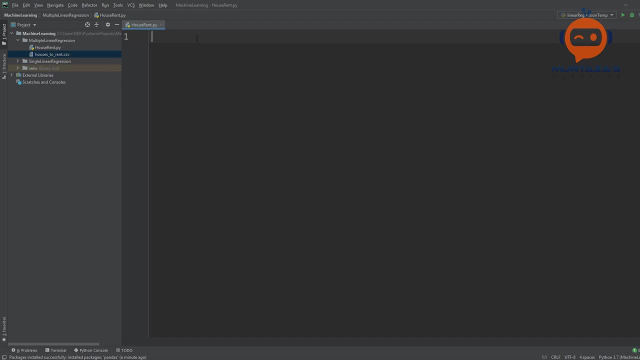 you're starting. so I will try my best to limit the number of libraries, that we limit the number of libraries, that we limit the number of libraries that we will be using so that we can easily will be using, so that we can easily will be using, so that we can easily understand and once we do understand the 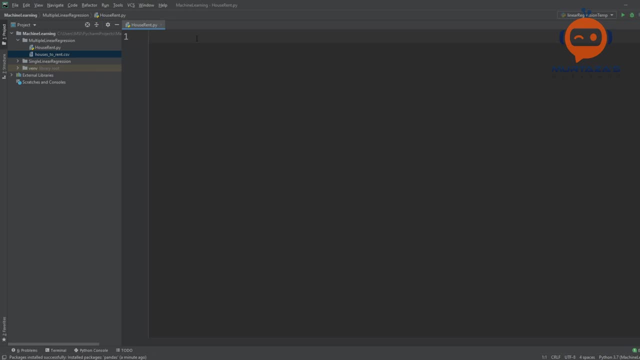 understand. and once we do understand the understand and once we do understand the basics, we can go into the next part and basics. we can go into the next part and basics. we can go into the next part and then try new libraries and some advanced. then try new libraries and some advanced. 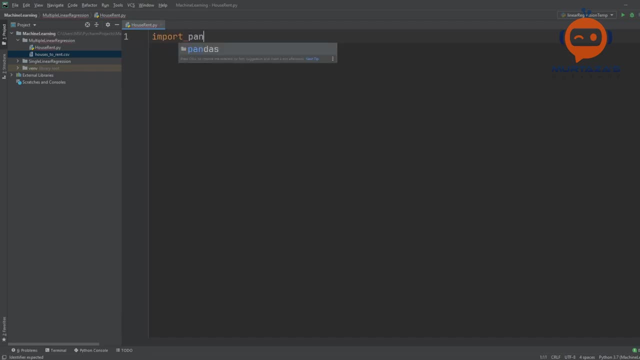 then try new libraries and some advanced stuff. so let's start with importing stuff. so let's start with importing stuff. so let's start with importing pandas. we are going to import it as PD, so pandas. we are going to import it as PD. so pandas. we are going to import it as PD, so that we don't have to write it again. 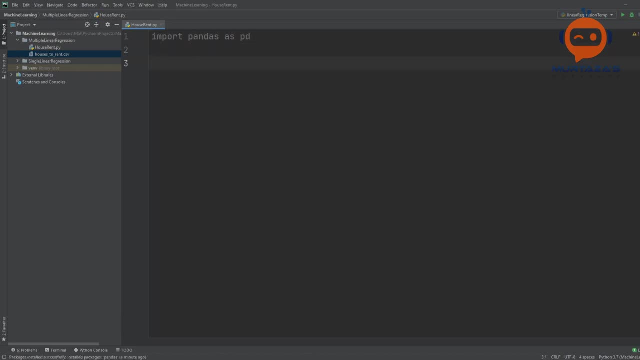 that we don't have to write it again, that we don't have to write it again and again as pandas, and the first thing, and again as pandas, and the first thing and again as pandas, and the first thing we will do is we will import our data. so 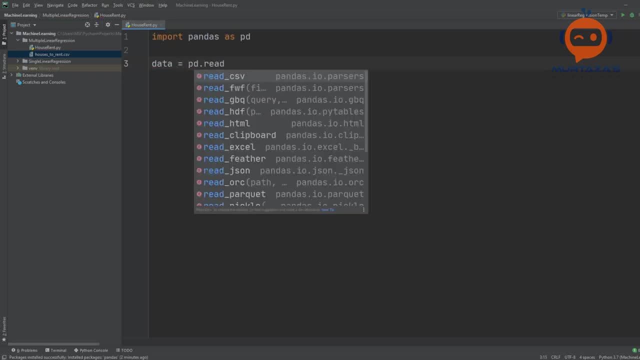 we will do is we will import our data. so we will do is we will import our data so data is equals to PD dot read and we data is equals to PD dot read and we data is equals to PD dot read, and we will write CSV and then we will simply. 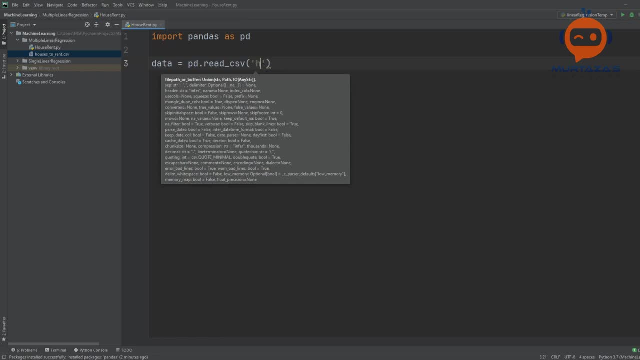 will write CSV and then we will simply will write CSV and then we will simply give the the name of the file which is. give the the name of the file which is. give the the name of the file which is houses to rent and we will define the. 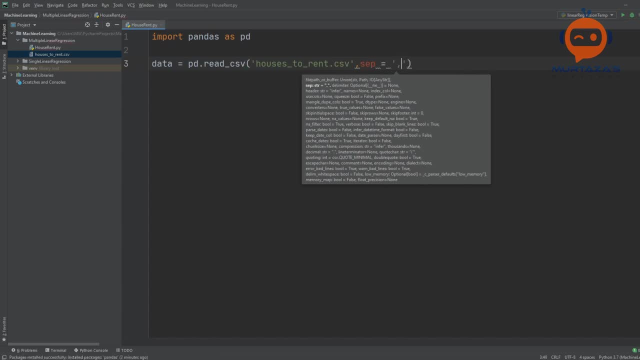 houses to rent and we will define the houses to rent and we will define the separation as comma. so this will separation as comma, so this will separation as comma. so this will separate the values for us- okay, and then separate the values for us- okay, and then separate the values for us- okay, and then we are going to define which of 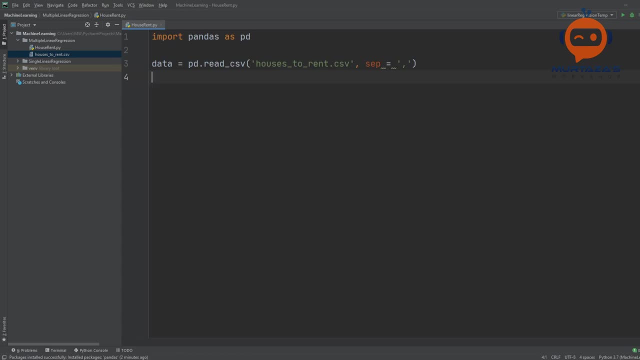 we are going to define which of. we are going to define which of these what you called values or columns, these, what you called values or columns, these, what you called values or columns that we want to use, but before we do that we want to use, but before we do. 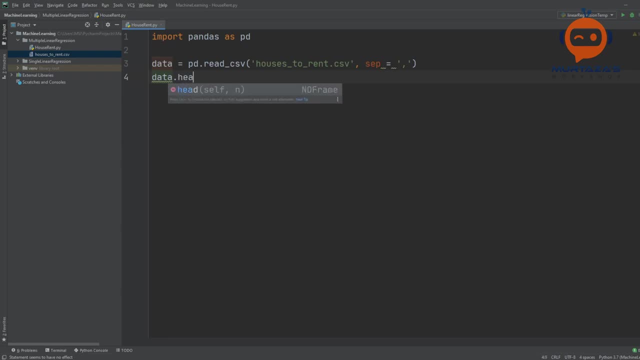 that we want to use. but before we do that, there is a method by the name head, that there is a method by the name head, so you can use this method to actually view the first five rows of your data. so this is a very useful method. so you can, right here, print and this will print out your data head. so if we run that, 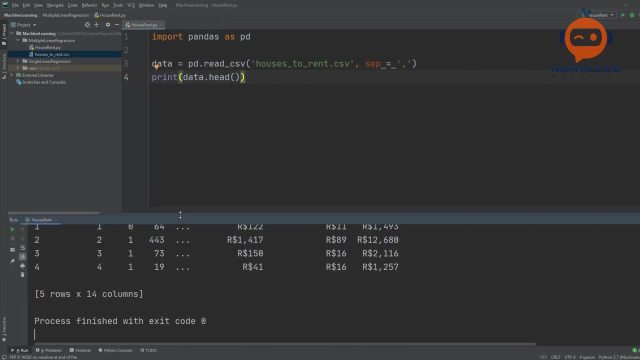 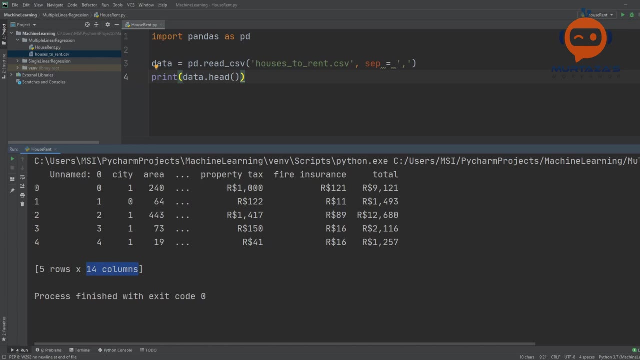 let's right click and run and there we have it. so you can see that it prints out the first five rows and you can see that we have 14 columns over here. so you have city, then we have area, property tax, fire insurance, total and so on. so this one is saying unnamed and it's repeating again. 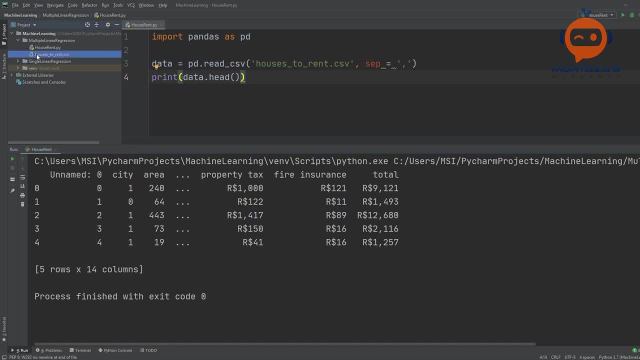 we can put id here, i think let's write id here and let's save that. and if we run that again and there we have it, so now it's not saying unnamed, so let's say this is the id and city and this everything else. okay, so once we have that, we are going to select the columns that we 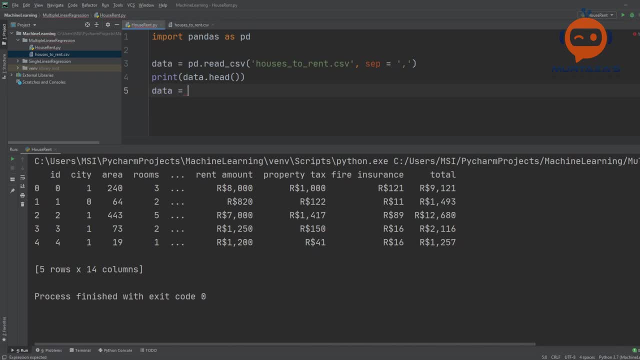 want to use. so we will say that data is equals to data, and then we are going to write all of the column names that we want to use. now there are two methods of doing this. now you can specify the number of the column so you can say, for example, 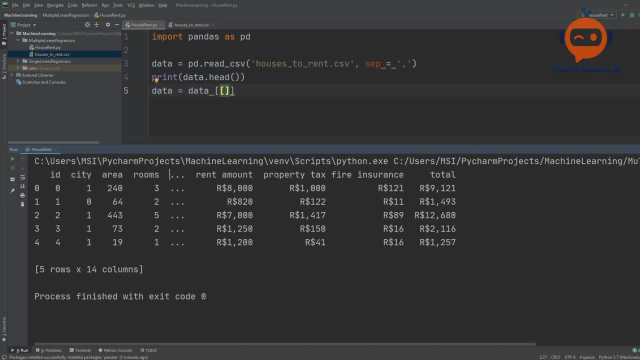 this is zero, this is one, so i want one, two, three, four, something like that. or the better way to do this is to specify the name at the heading, so that is a better way to do this, because it will be easier to see what is happening, so we will be using that. so here, for example, the first one: we 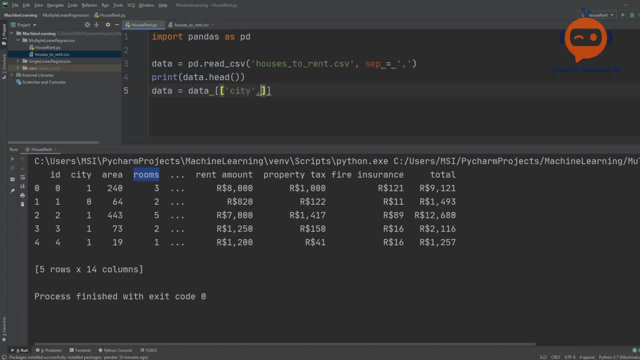 will write is city, and then we will write rooms, rooms, and then we are going to write bathrooms, bathrooms, bathrooms, bathrooms. is it rooms or room? it is room, not rooms. and again it has to be exactly the same. so if i go back here, it says bathroom, so it has to be bathroom, not rooms. and then we have parking. 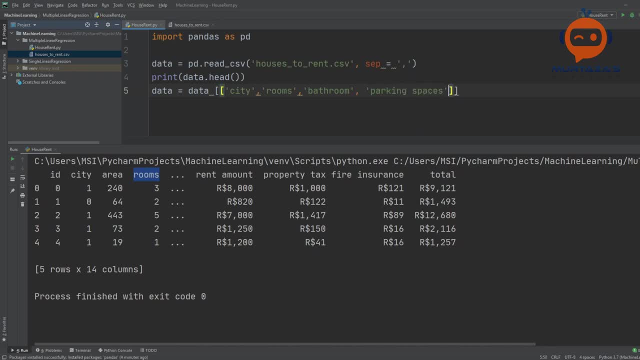 spaces, spaces. so here i have randomly selected some columns. you can choose your own as well. so here is fire insurance: ranc, oxa zero. so let's go up91 nce. and it's getting big, so let's go down, and then we will write here, let's say, furniture. so what i've done is i have mixed up the 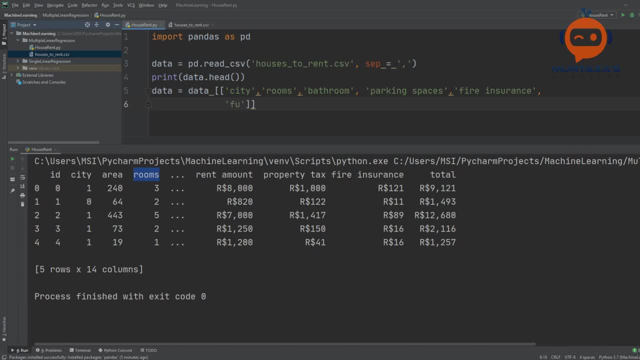 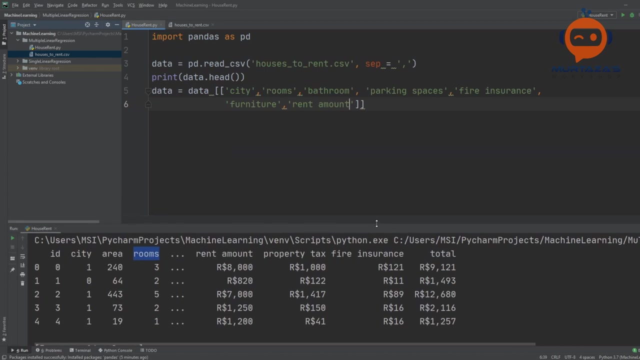 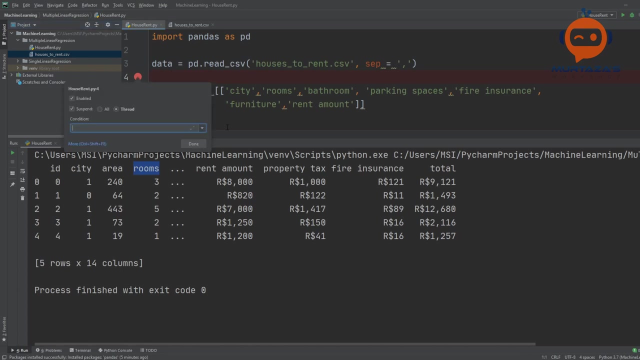 type of data we have. you will see later on why. because we want to see all the kinds of data that we can have, so we know how to use them before, how we can filter it before we send it to the model. so we will write furniture. And the last one is the one that we will be using as our output, which is, in this case, the amount of the rent. So we will write here: rent amount. So this is it, And again, we can just take this and we can cut. Let's remove the break. 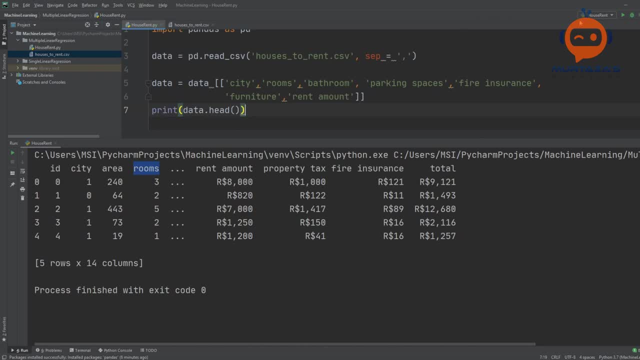 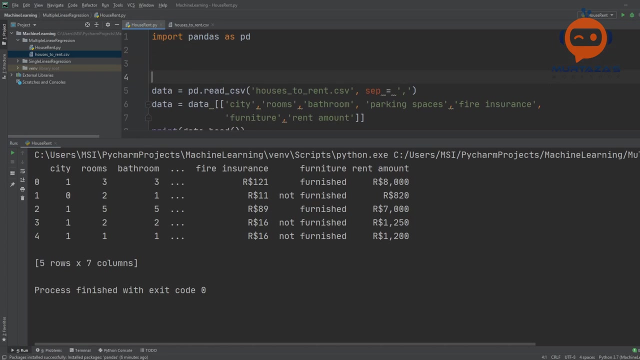 And we can write here and we can print. So now you can see that right away. it has become again it's five rows, but now we have seven columns. So it's city rooms, bathroom, fire insurance, furniture and up till rent amount. So that is good. Now this whole area. we can call this as loading the data. So it's better to write comments, So load data. 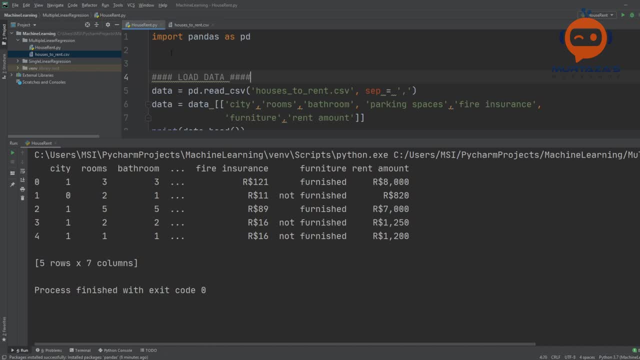 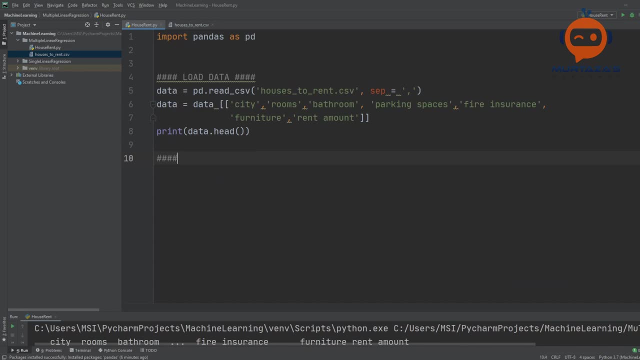 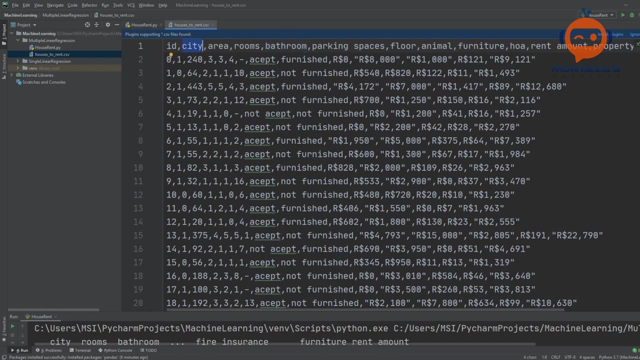 So that is done here, And let me just bring this down so it's easier to see. So the next step is to actually process our data. So we are going to write here: process data. So what kind of processing do we need? So if we look at our data here, So you can see that the city is basically already they have, they have converted it into one and zero, So we don't have to. 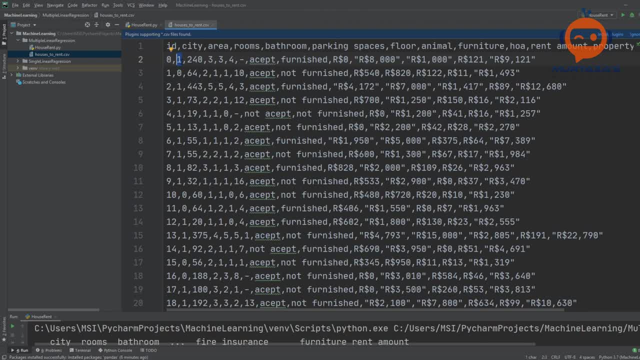 do anything over there. So city means one means it's in city, Zero means it's not in city And but for, for example, furniture, it says it's furnished and not furnished. So we need to convert this into zero and one, because the machine learning model does not understand strings, It understands numbers. So we have to convert this into zero and one. In the same way, if we had different cities and we had the names of these cities, So we will have to convert these names. 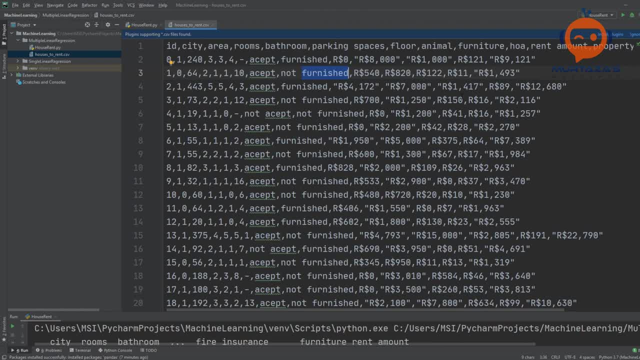 To zero: one, two, three, four. For example, zero means New York, One means London and then two means something else. So all of these will be categorized into numbers rather than strings. So this is what we have to do, And the second thing we have to do is we have to remove this RS, and we have to remove any of these- what do you call commas as well. So this is what we have to do. So the 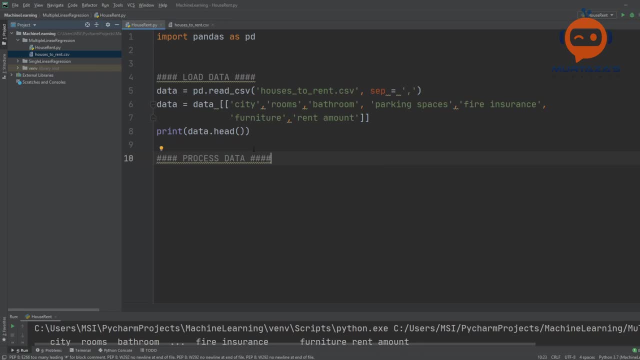 is all of the processing of the data, that, uh, that we have to do so. there is a method within our pandas library that is associated with the data. so what we are going to do is we are going to use the map function to actually solve this problem. so it's very simple. it's just one line of code. so 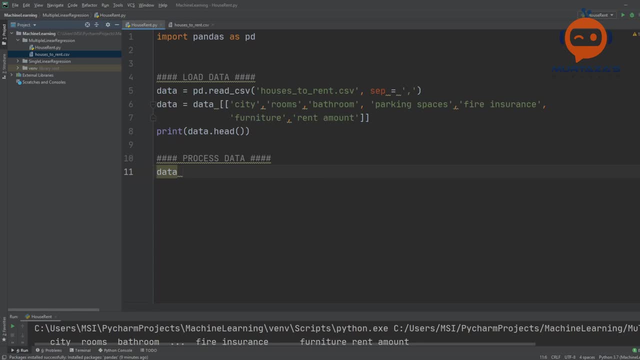 we will write here data. so first of all, uh, what should we do? let's do the rent first. so let's write here rent, rent amount. so this is what we are talking about. and then we want to change our data at rent amount, rent amount. and then we are going to use that method, dot map. 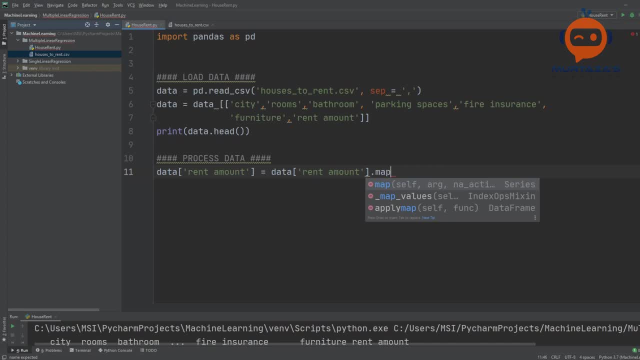 dot map. this means that, using a function, we are going to change all of the values within our- uh, what do you call data- rent amount. so here we are going to write lambda. now, lambda is basically a single line function so that you can write, and it does not have a name. so what we are doing is basically, we are saying that 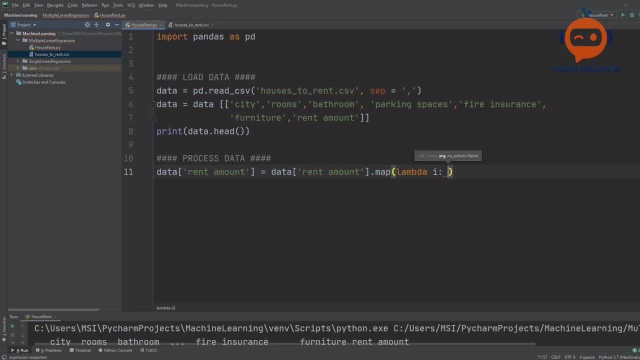 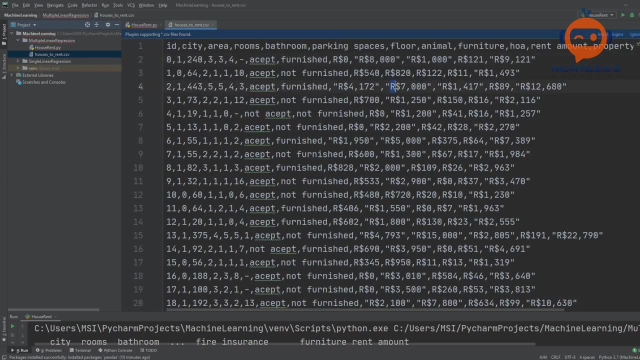 this is our variable i. we are saying that we want to take in the first two. let me just show you here. so what we are saying is that we want to take out these first two elements. so this will be 0 and this will be 1.. so we want to remove this element. so this is basically a string. 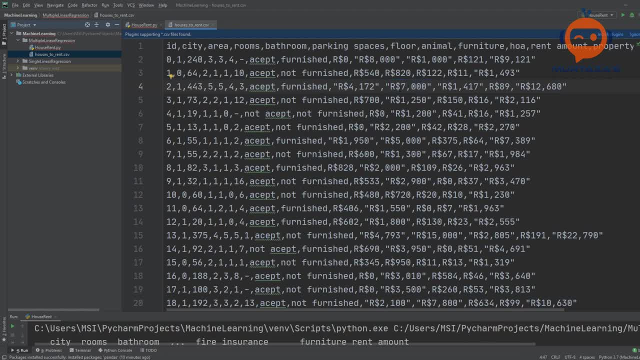 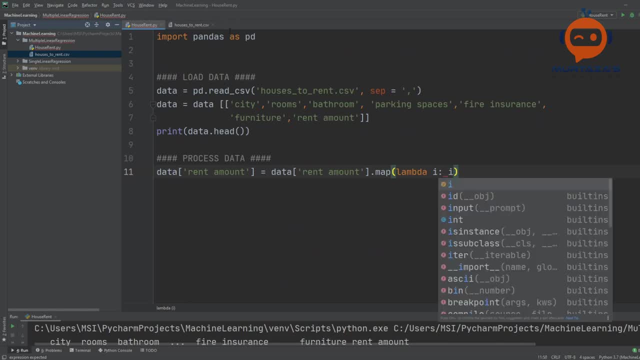 so we can use the slicing function of the strings to actually remove this. so we are going to say that we want to remove the first two elements. so let's say this value that we are talking about, this 7000 value is what we are getting. so this i will be the 7000 value. so we will say that we want. 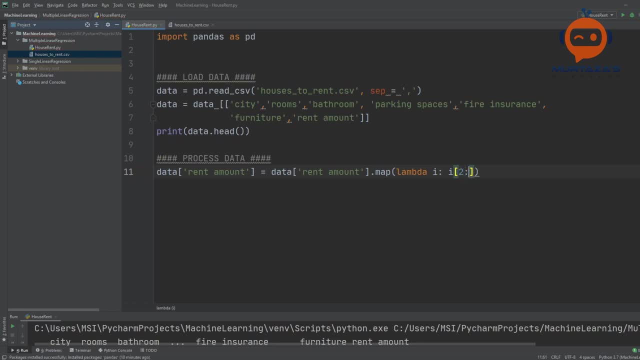 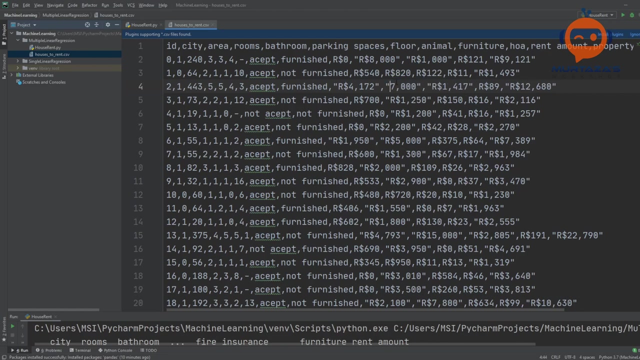 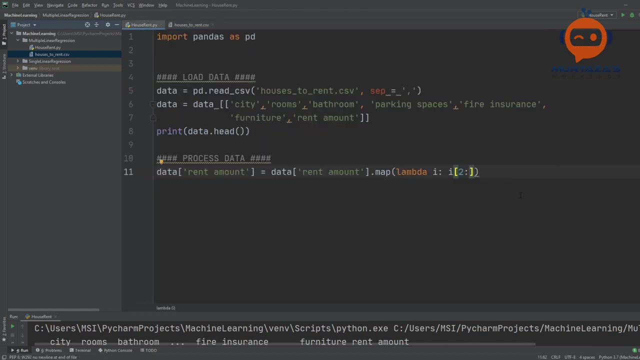 to remove the first two values, so we want to start from two and in the end, we are not giving any value. so this is what it means, and then this will replace: uh, this will remove these two things. okay, but we still have this. so to remove this, we are going to use the replace method, so we will. 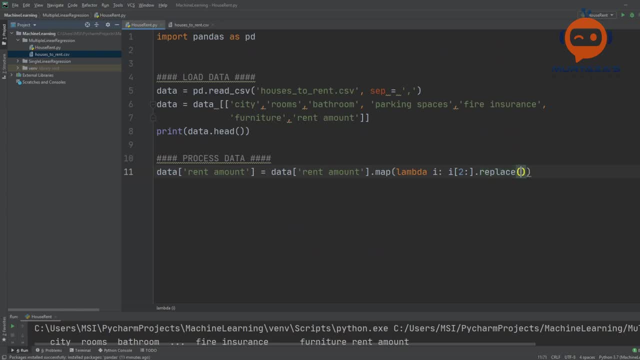 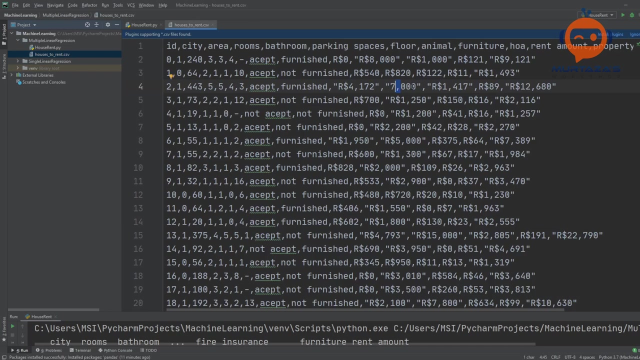 write here: replace and to replace. we are going to say that we want to replace a comma with an empty space. so that is how simple this is. so here we are talking about a single value. so that means if, for example, we have some functions, and if we have some functions that we want to. 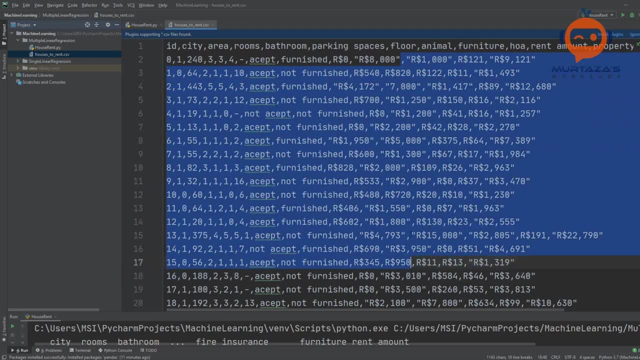 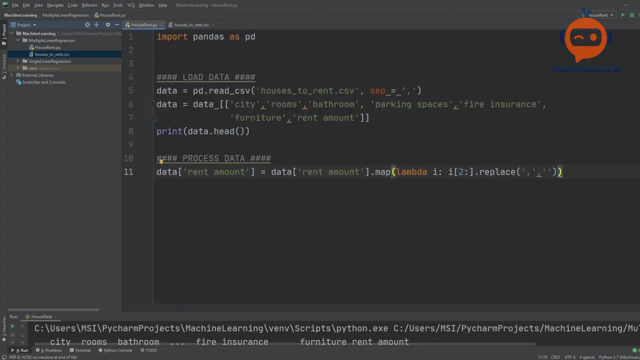 itezred an empty blocks or some things, and if i want to Gewвин some things. so what i want to do is I'm just going to call this hashtag thing and I hand it in here to the class variable. so, all right, let's see what I can do. so this is a different method, so let's see we are going to. 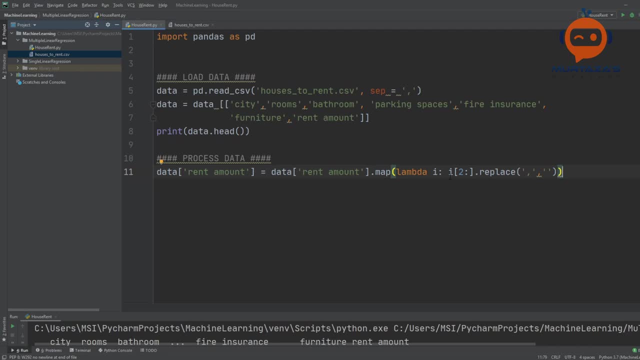 have that loop function. we are going to type like this, right, so let's assume that this is our okay, so that is good. but the last thing we have to do is we have to convert it from a string to an integer, because we are talking about numbers, so we will convert it into a string- sorry, a number. so 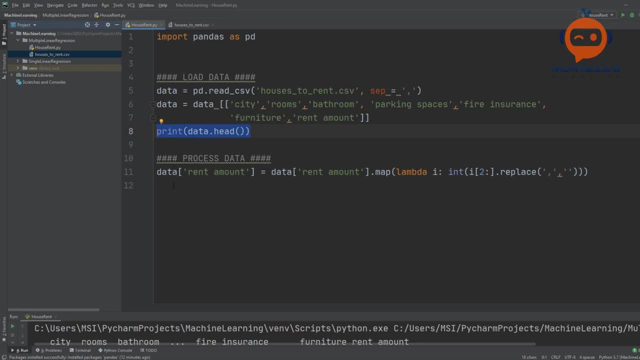 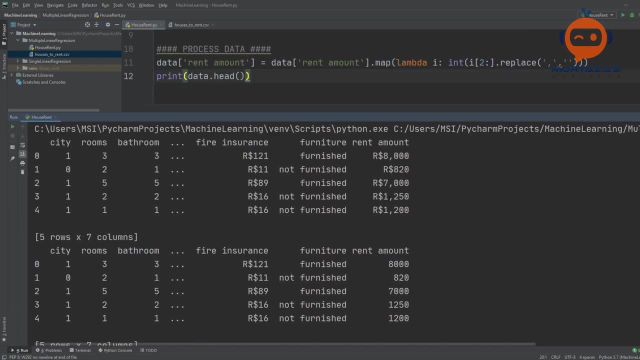 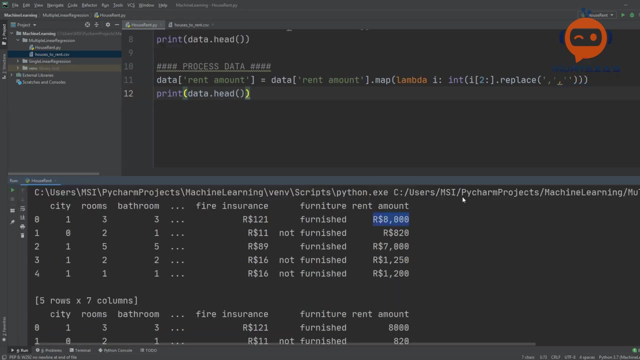 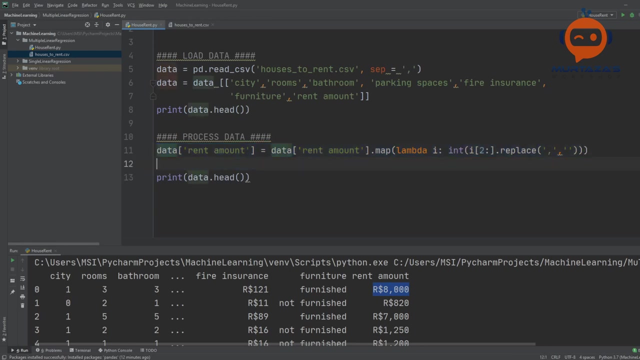 let's print out the head now and let's run it. so there you go. so now it's converted back. so here you have 8000, here it was rs8000. so if i don't do, let me just copy that and let me paste it. oh, let me paste this here. and if i don't do, 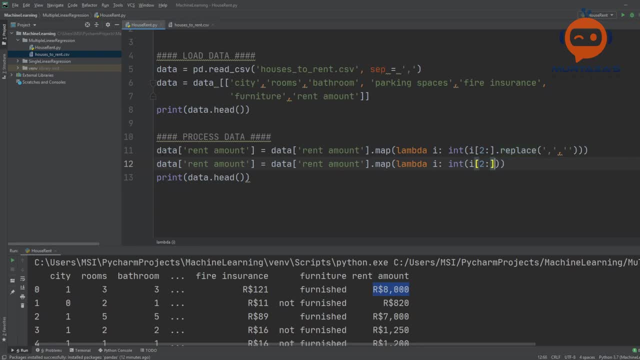 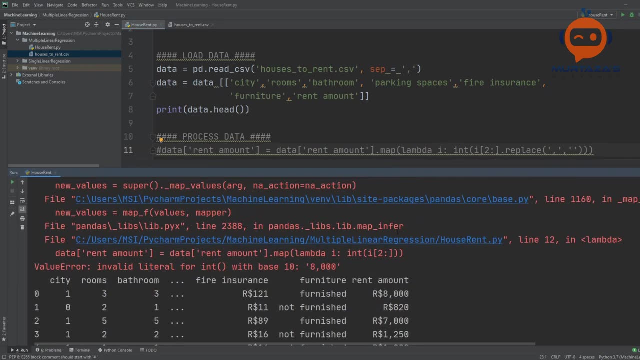 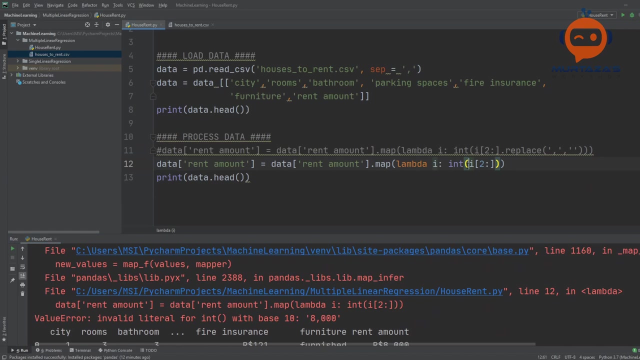 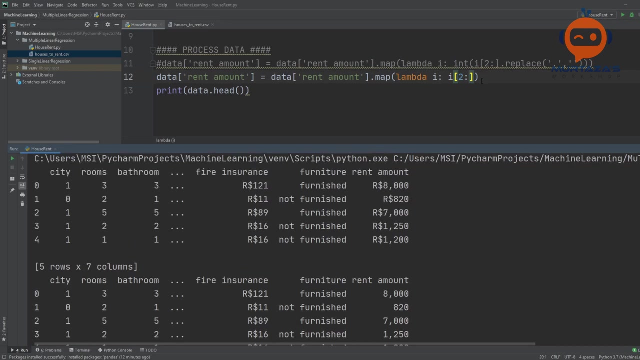 the replace parts, you can see: oh boy, there is an error. oh yeah, you cannot convert it if you did not actually change it, so let's do that. uh, okay, so here you can see: if we don't do the replace or the integer, then this is what we get. 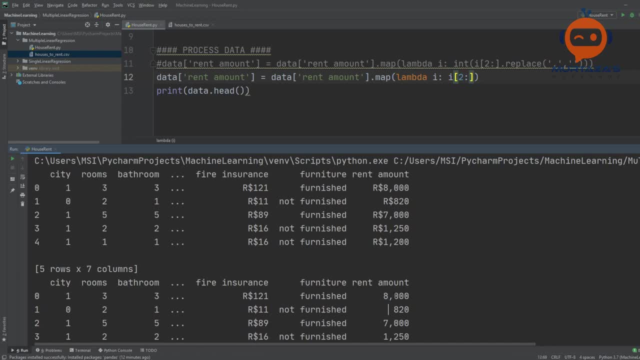 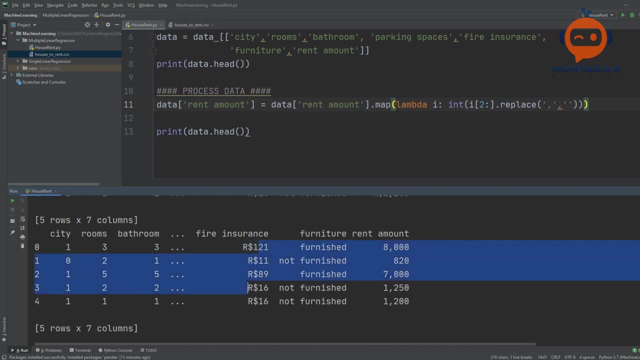 so first we are basically removing the first two values, and then we are replacing the comma. so this is what all of this is doing. so this is for part one, and then we also have to do for the fire insurance. so we have to do the same thing for the fire insurance. 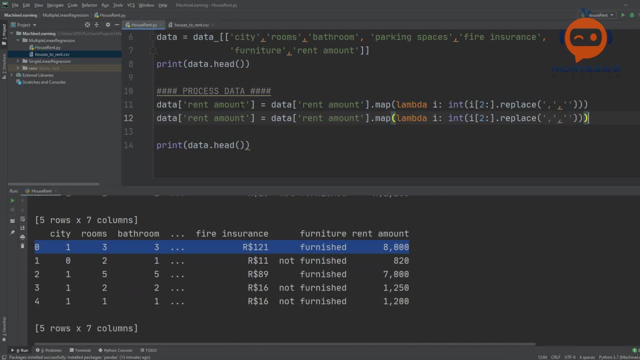 so we can simply copy and paste this. if we have a lot of these, we can put it in a loop, but in this case we don't have a lot, we only have two, so i'm not going to put it in a loop. so let's do this and let's do it here. 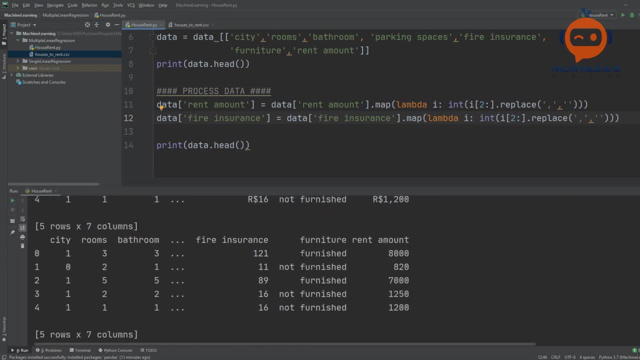 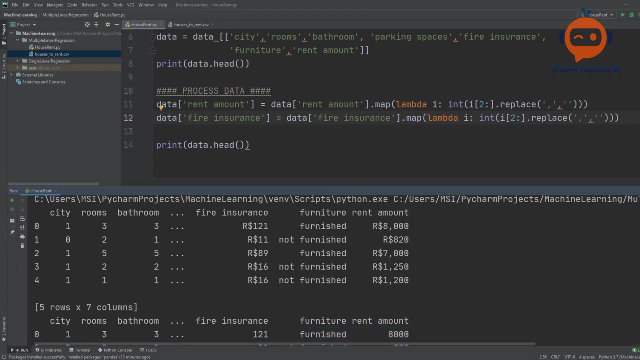 is it visible? yes, it's visible, so let's run that, and there you go. so now the values. earlier we had rs one to one and now we have one to one. so that is good. and the next thing we have to do we have to change the furniture, uh, but from furnish not furnished to zero and one. so to do? 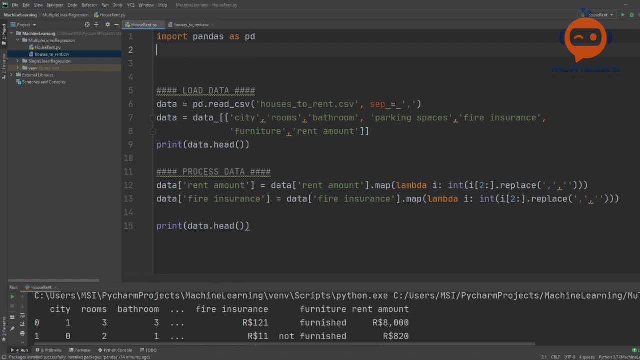 that we have a function in the scikit-learn, so we are going to import- uh, let's write from from sk learn imports. we are going to import pre-processing, so here we are going to just define the object. le is equals to preprocessing, dot label encoder. so this is our class. 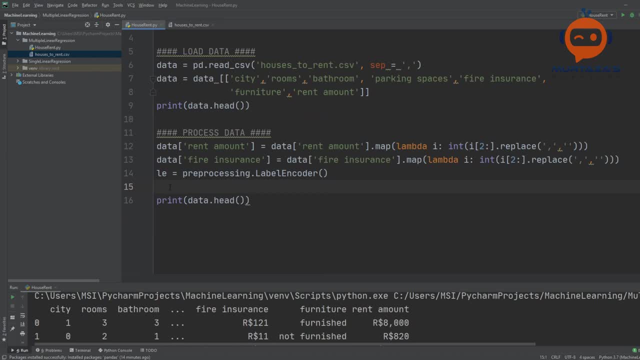 and what we will have to do is basically we will write here again that data we are talking about. this time we are talking about the furniture for nature. did i write it wrong? no, it's fine. so furniture. and then we will say that le dot fit, and we're going to fit transform, and inside we are going to write this again. 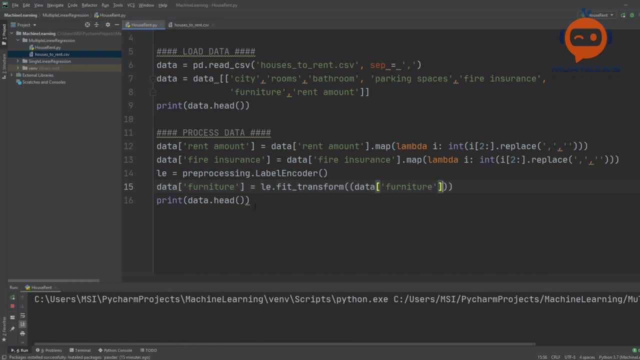 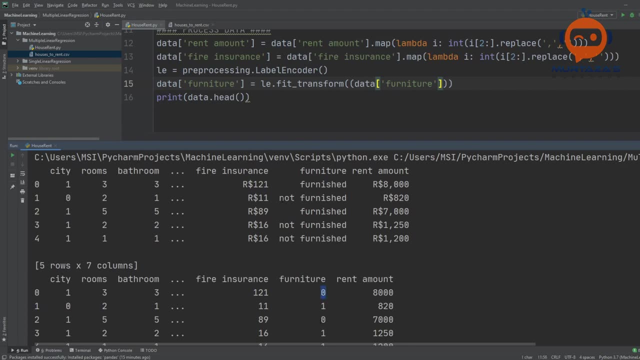 data furniture and if we run this now, so the first thing we are going to do is this: we are gonna call it, not furnished. this is our data that weνη called le ban totally, and we all know what it is, so now it's showing us how to whitewash it, what they store the data in and what we need to say.